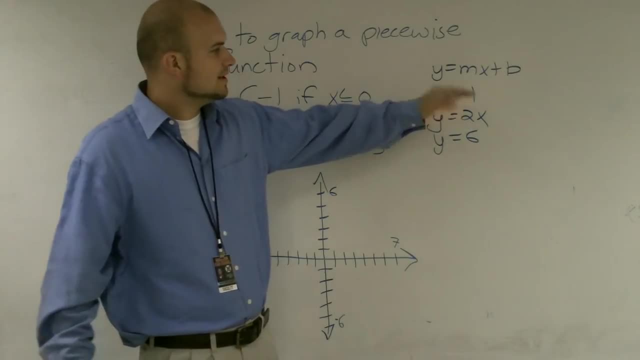 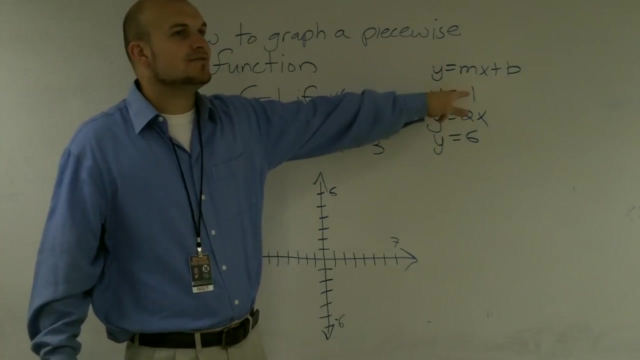 and then what is going to be the slope? If I look at this first one, I notice that there is no x, so therefore I have no slope And my y-intercept has got to give me a negative 1.. Therefore, this is going to be a constant line at negative 1.. Now, when graphing a linear 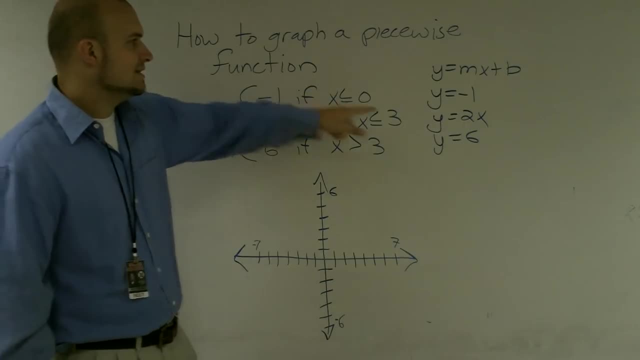 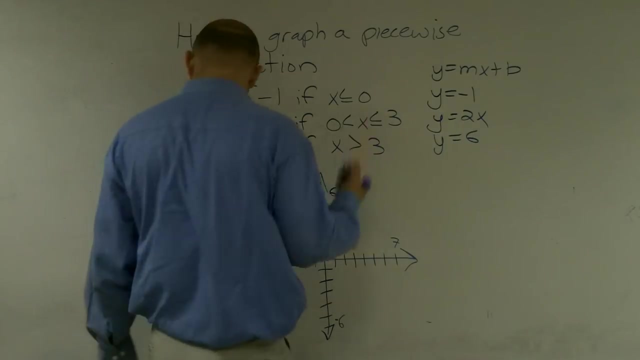 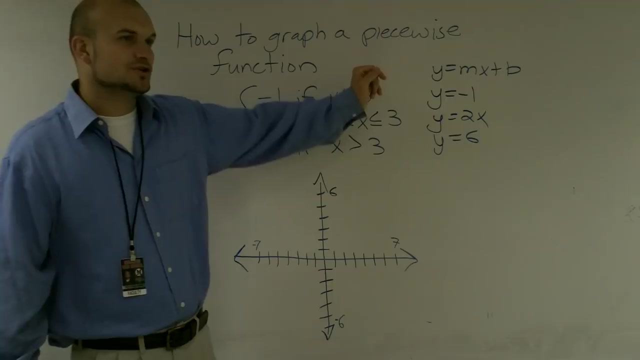 equation, I notice that I have constraints. This graph is only true when x is less than or equal to 0.. So what I can do? there's a couple of ways you can do it. You can just graph it as when it's only true. or you can maybe just graph the whole equation and then start erasing. 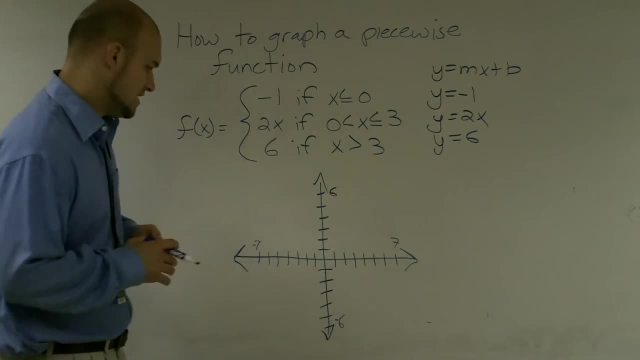 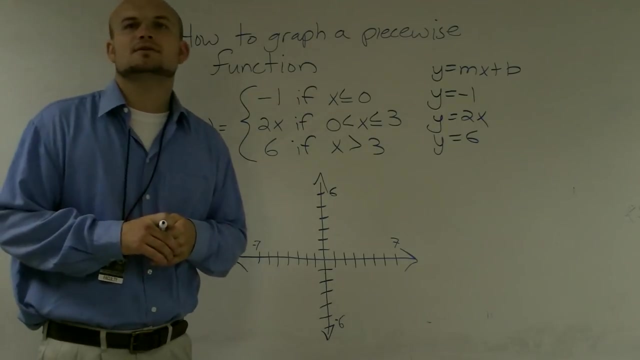 where it's not true, And I'm going to go through that just so you guys can kind of see what the whole graph will look like. So I have x equals negative 2.. Actually, Samantha, could you look at my? actually you can see. 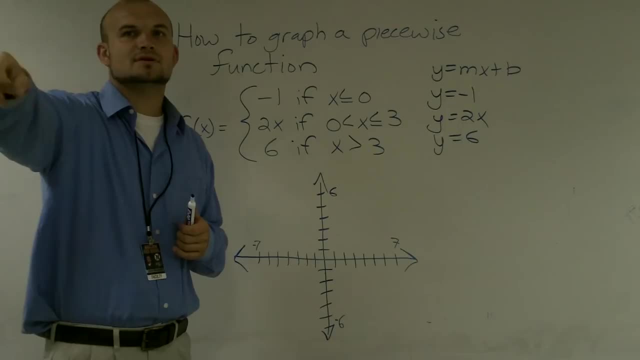 that red marker right on the, in the folders, in my folders, in my folders to the right, You see a red marker. Yep, you just throw it Well underhand, toss it. You know you're making a video right. 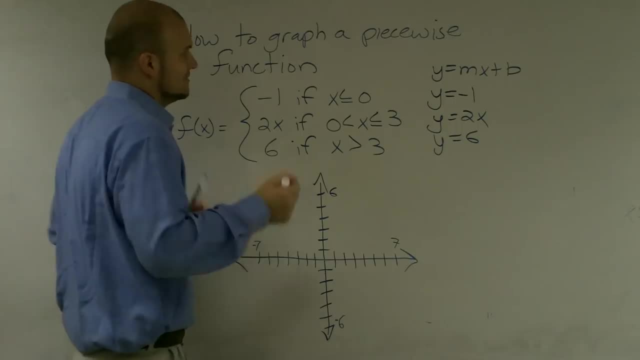 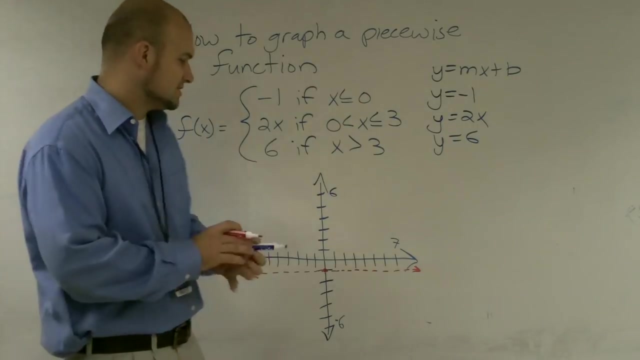 I know, I know, OK. So if I was going to graph this at negative 1, I'd go down to negative 1.. All right, Then I'd now say: all right. it's only true, though, when x is less than or equal to 0.. 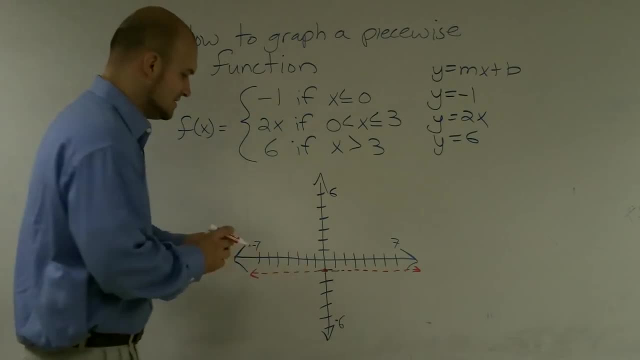 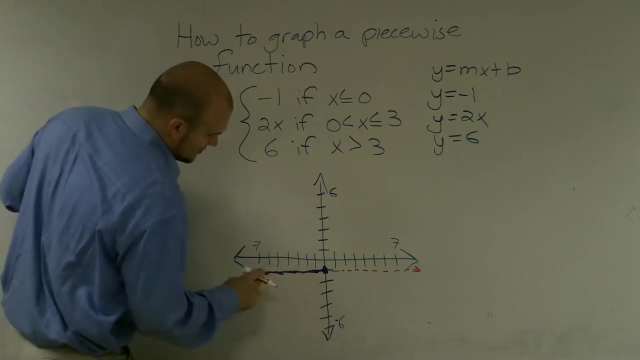 Well, where it's 0, where x is 0 is right at the y-intercept. So therefore, this graph, I'm only going to shade in where it's true, We're not going to shade, we're not going to draw. where it's false, We don't care about where it's false, We only care about where. 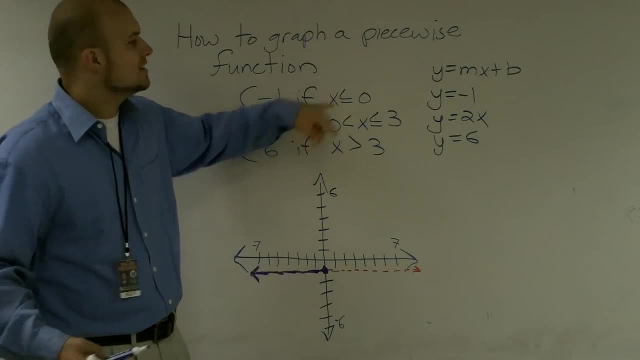 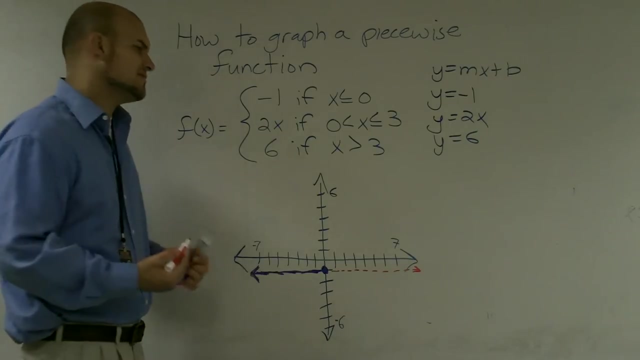 this equation is true, So it's only true when x is less than or equal to. Since it's equal to, it's going to be a closed circle. Next point: y equals 2x. What does that graph look like? Well, I know that. my slope now. 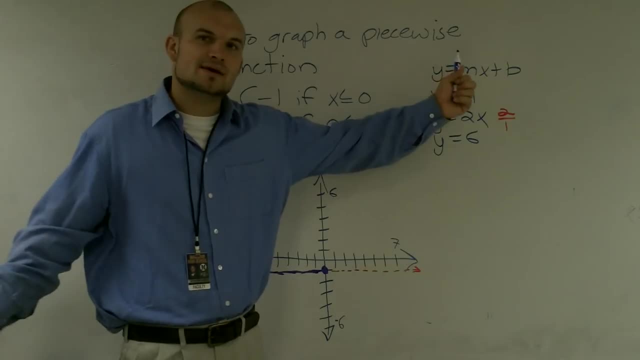 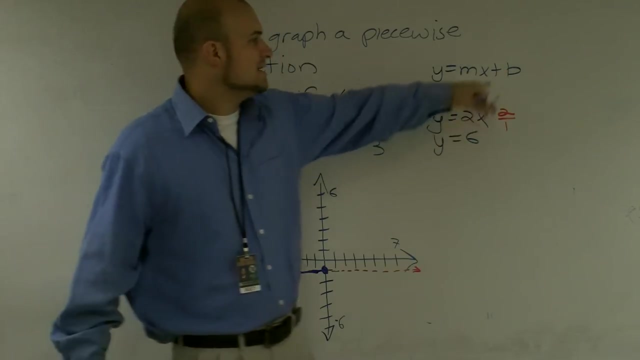 has a slope of 2 over 1. And I do not have a y-intercept. I'm sorry, my y-intercept is 0, since it's not labeled up there. So I do have a y-intercept at 0, but it's not shown. 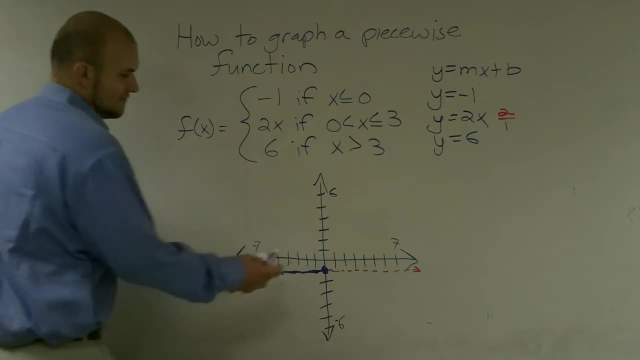 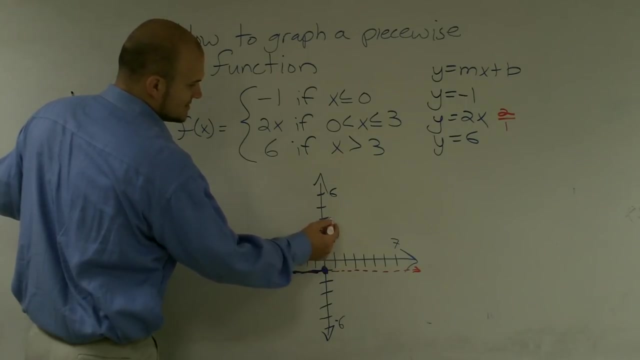 in the equation. So therefore I know it's 0.. So therefore, on this, to graph it, if my slope is now 2 over 1, that means I'm going to rise 2, go over 1.. Rise 2, over 1.. So now we're down 2 to the left 1, and down 2 to 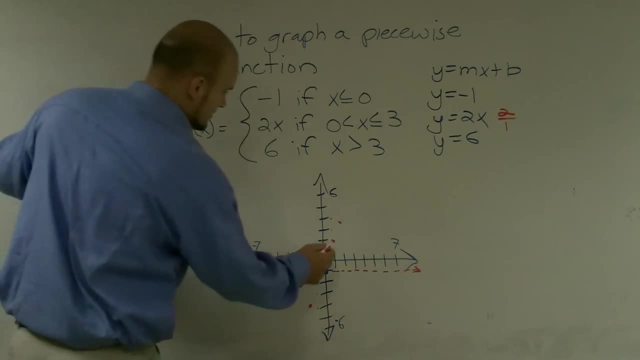 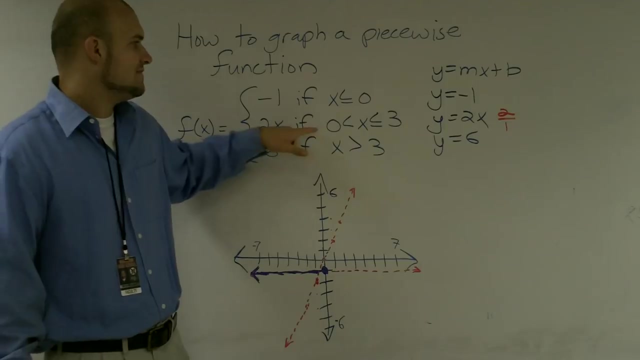 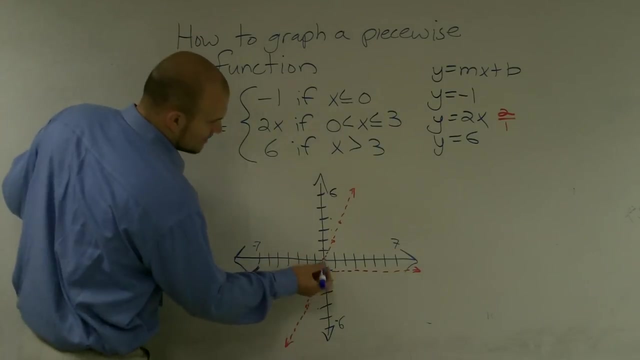 the left: 1.. So, again, I'm just going to dot a line, just so I know, just so I approximately know what my graph is going to look like. Then it says this: however, this graph is only true from 0, when 0 is less than x, or less than or equal to 3.. So therefore, since it's just 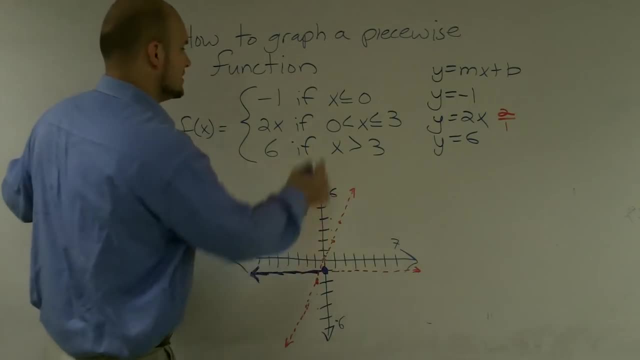 less than I know it's going to be 0.. Since it's just x is greater than it's going to be an open circle And it's going to be between 0 and 3.. So I'm going to go over 3, 1,, 2,, 3.. And I'm going to follow that up to. 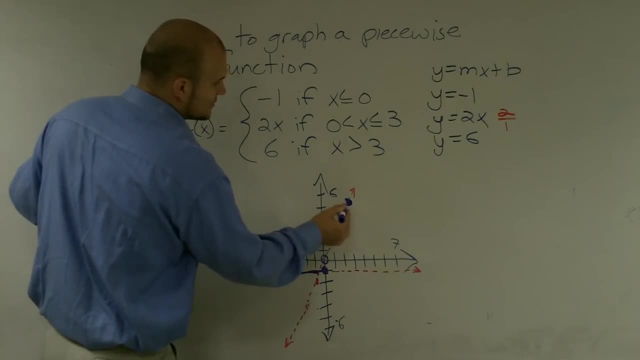 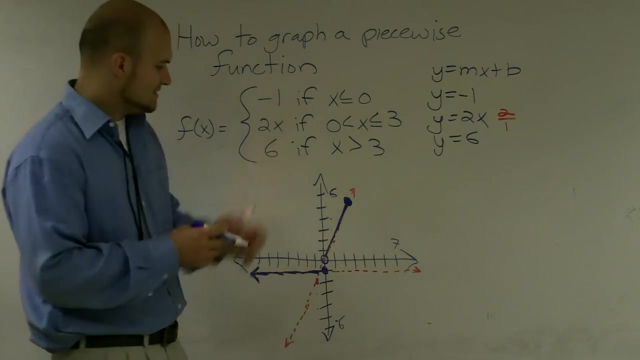 my graph, And now this is going to be, x is less than or equal to 3, so it's going to be a closed dot And I'm just going to shade in this graph here. So that is between 0 and 3 is only when this equation makes sense. That's the only time that equation is true. 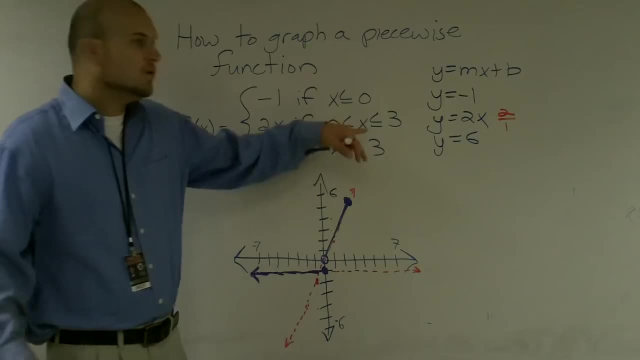 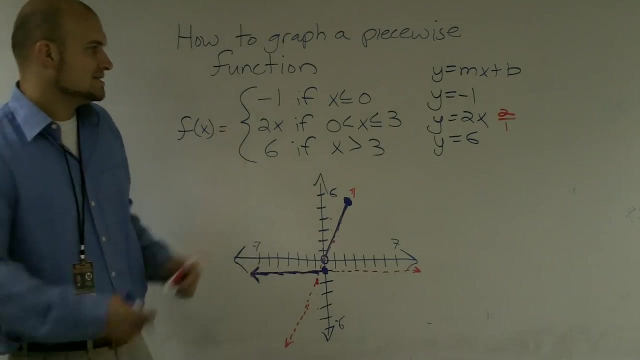 All these. this value is over here and these values are over here, So I'm just going to go over here. It's not true under these constraints, So I'm not going to include them in my graph. And then, lastly, I have y equals 6. Again, it's just like y equals negative. 1. The y: 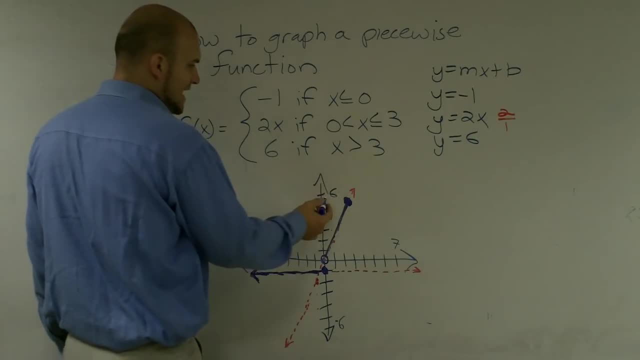 intercept is at 6. And it says it's only true when x is equal to 0. Or, I'm sorry, x is greater than 3.. So therefore, at 3 again, I'm at all right, my 3.. 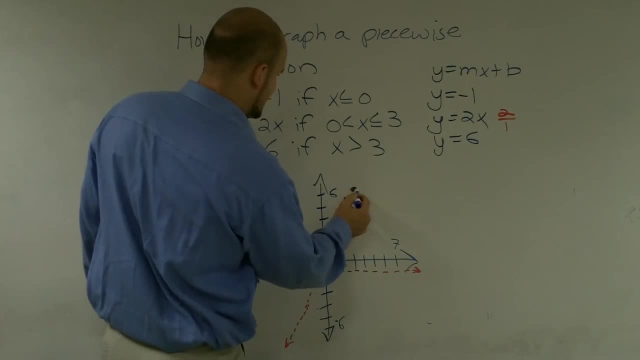 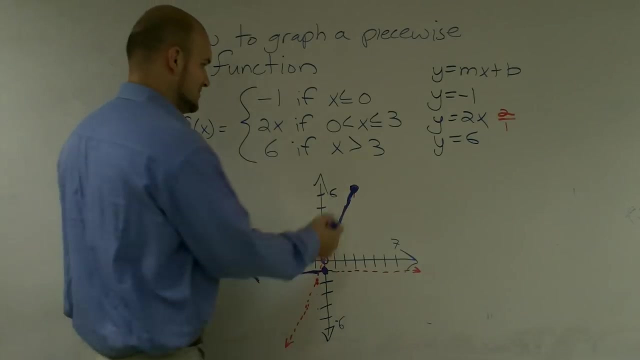 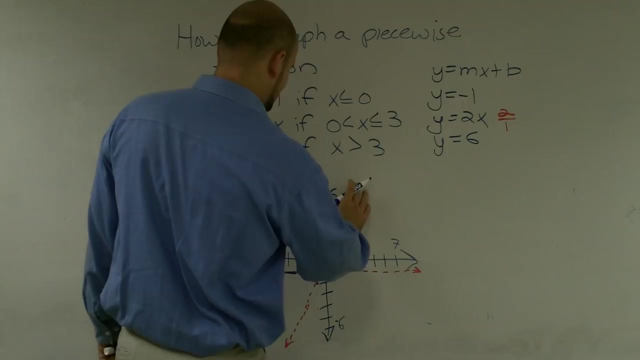 That dot really should be about there. Sorry guys, I don't have graph paper on my board, so I got to be close to as proximal as possible And x would be at 3.. 1,, 2,, 3. And x greater.